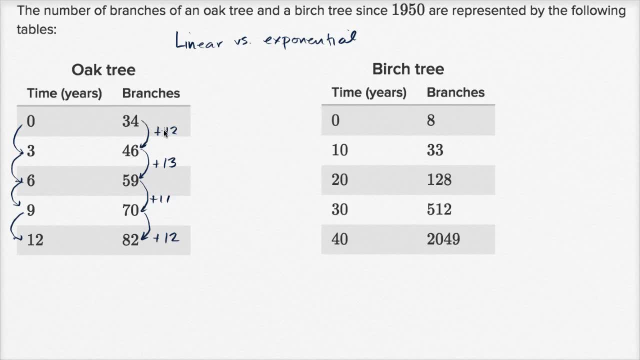 of the behavior of the number of branches over time. For me this is pretty close to a constant 12 branches a year. So I would construct a linear model here. I would say here Here: branches as a function of time. Let me be clear. 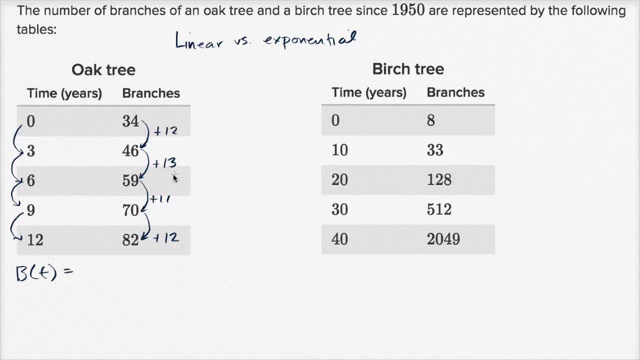 This isn't 12 branches per year. This is 12 branches every three years. 12, this is 13 branches over three years. This was 11 branches every three years. We're going to average 12 branches over three years. 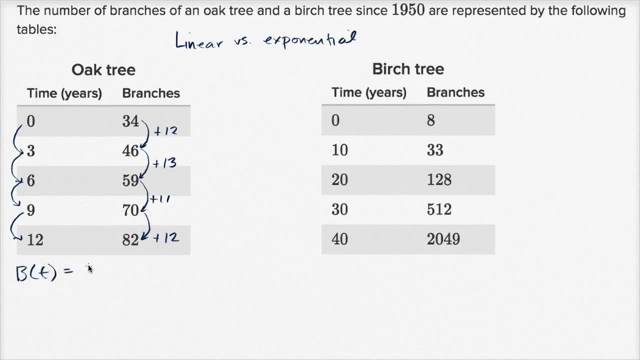 So the number of branches we have, we're going to start at 34 branches And then minus. if we have 12 branches every three years, that's four branches every, or I should say plus four branches Every year, And you could test this out. 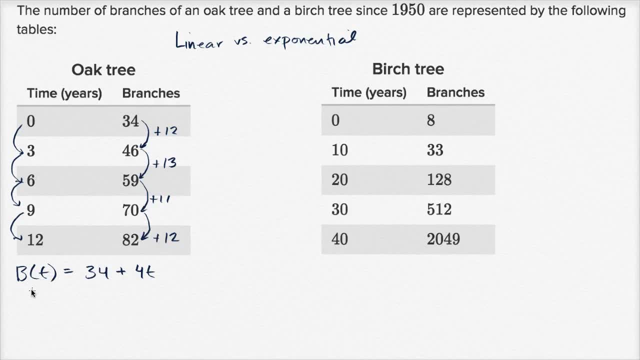 B of zero is going to give us 34 branches B of 12, let's just really test out. the extreme part of the model B of 12 is going to be 34 plus 48, which is equal to 82.. 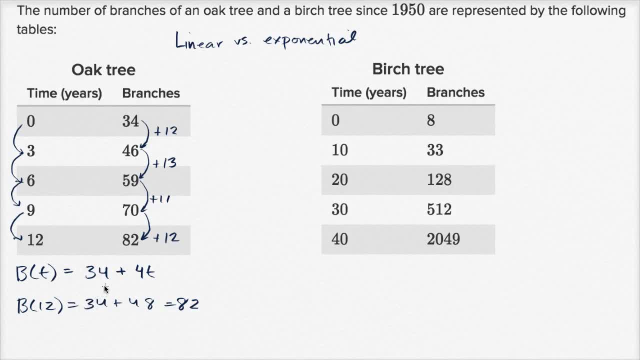 So this model works quite well. It's going to have a couple of places where it's not exactly fitting the data, but it fits it quite, quite well, And so this is a linear model. So this one is linear. Now let's look at the birch tree. 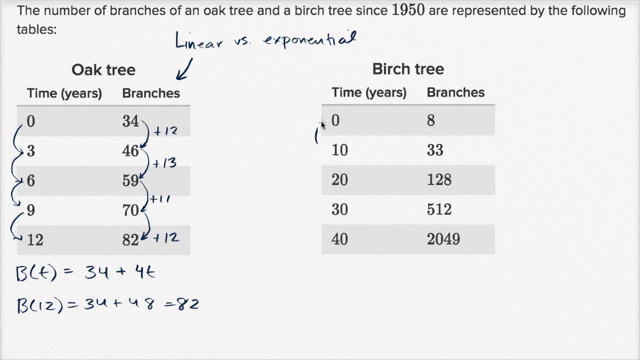 So time equals zero. so fixed change in time. Maybe I'm on the wrong layer, All right, so we have a fixed change in time every time we are moving into the future, a decade. Let's see our change in branches. we go from eight to 33.. 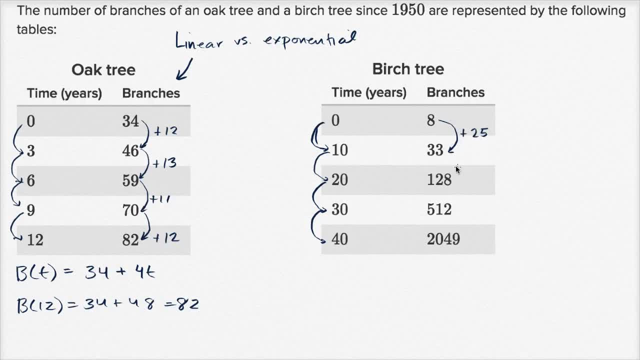 So what is that? That is plus 25 branches. Then we go from 33 to 128. Well, that's way more than 25 branches. That's going to be what? Five less than 100.. So that's going to be plus 95 branches. 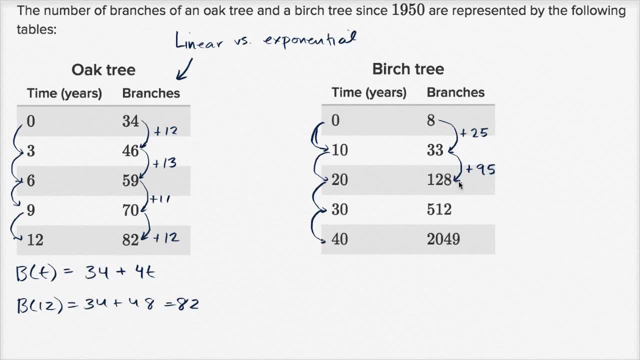 So this clearly is not a linear model, And so let's think in terms of an exponential model. How much do we have to multiply to go from? did I do that right? 128 minus. yeah, if it was 133, then it would be 100,. 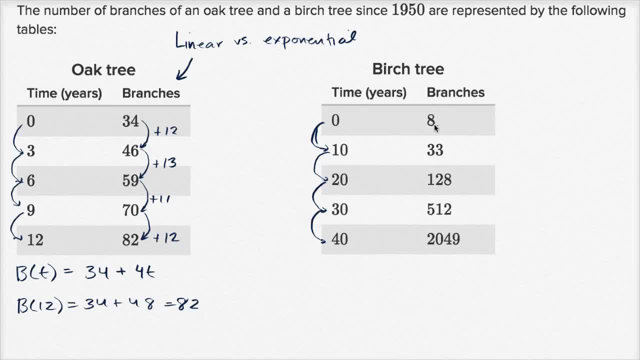 and then it's five less than that. yep, okay. So now let's think about it in terms of an exponential model. In terms of an exponential model, we care well what do we have to multiply for each step? So, if we have a constant step in time,